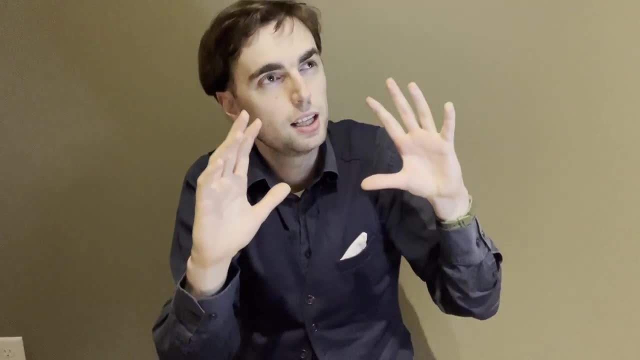 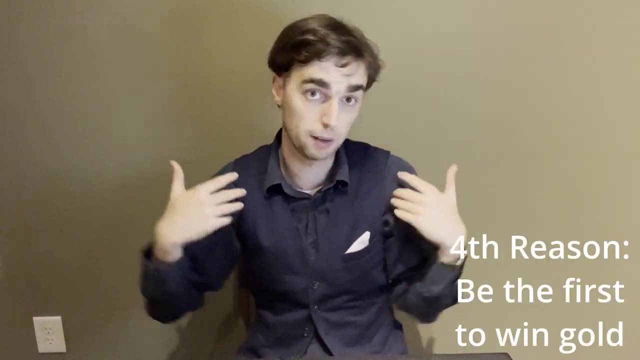 changed that. I saw it as a thing that could be a stepping stone to further and further success. Now I also wanted to be the first person in my country to win a gold and to win a gold medal. I wanted to be the first person in my country to win a gold and. 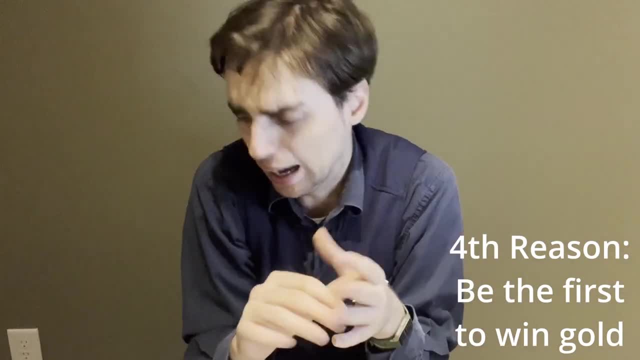 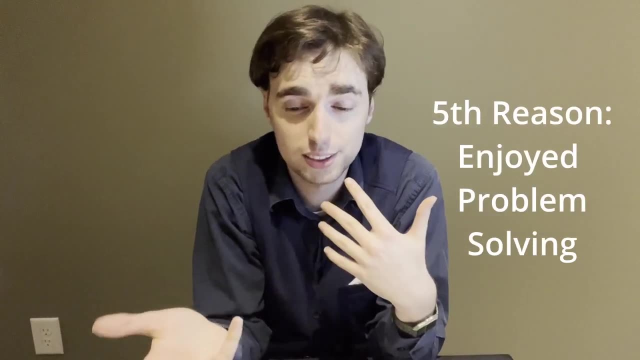 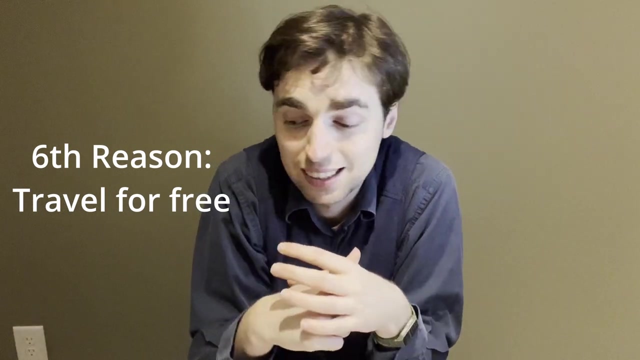 international math olympiad, which I failed. After a while the goals shifted again and I just did because I enjoyed problem solving, I enjoyed the whole process and I could also travel, potentially to a location at where the IMO is and have fun, enjoy myself. Now, there was one thing I didn't. 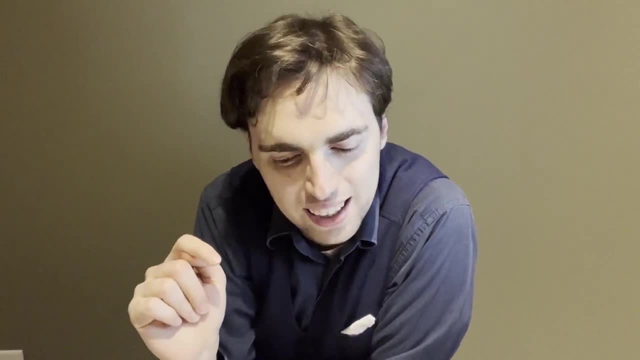 really know until after I finished competing and in fact until after I'd gone to college- that I realized was a super important thing. I didn't really know until after I'd finished competing and in fact, until after I'd gone to college that I realized was a super important reason. 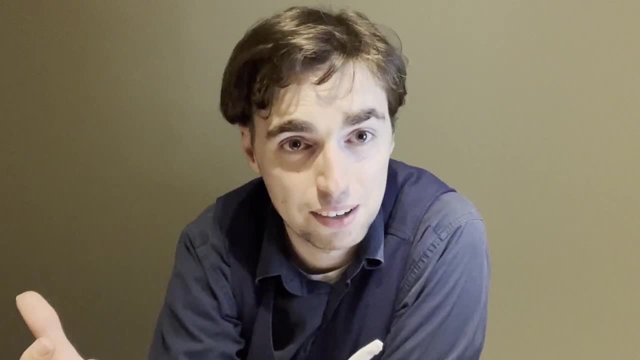 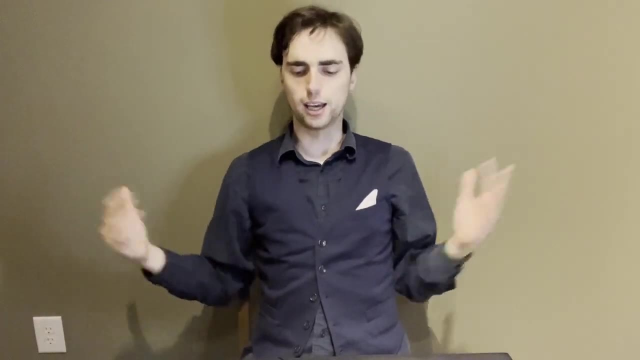 for why I should have done more and more of competitive mathematics, and I will mention that very important reason at the end. Now we go to the next question after we've answered: oh okay, why are we doing this? The next question is: what else can you do If you're saying no to? 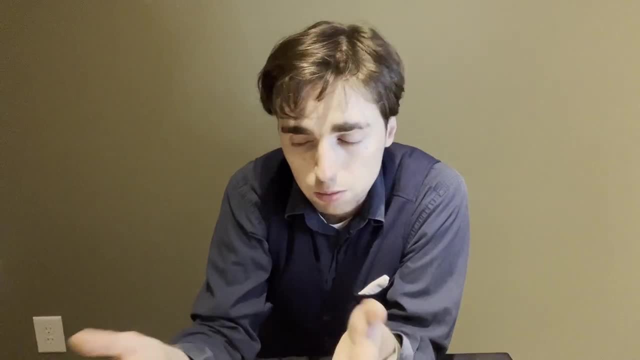 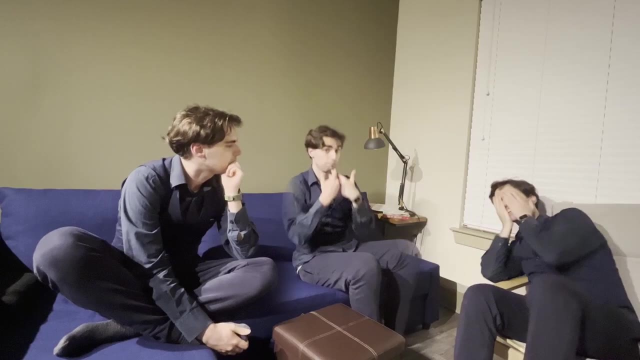 competitive mathematics. the question is: what are you saying yes to? Is it learning to code? Is it maybe learning to become a professional chef, Learning how to play music or just enjoying life with friends? What are you saying yes to? Is it maybe learning to become a professional chef? 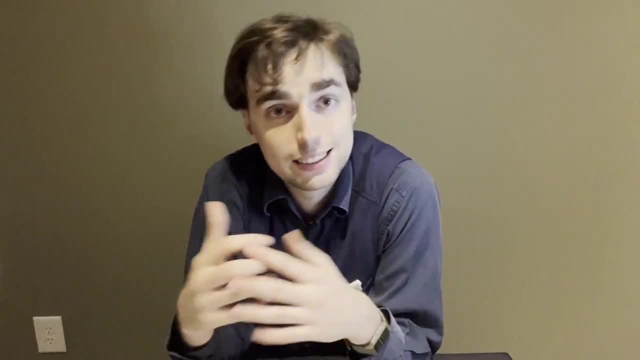 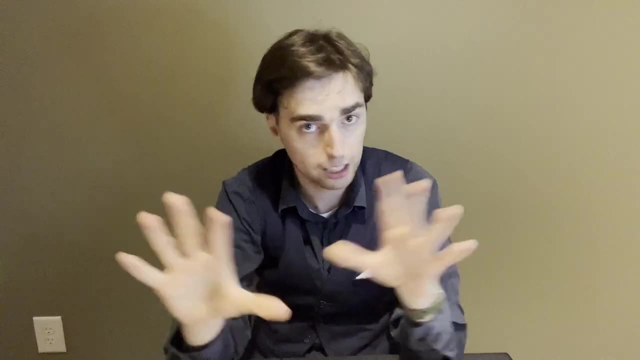 Learning how to play music or just enjoying life with friends? What are you saying yes to? Is it that you actually would like to do instead? Now, before we move on to the third and maybe the most important question, I need to give you some things you need to know, and the first thing that you 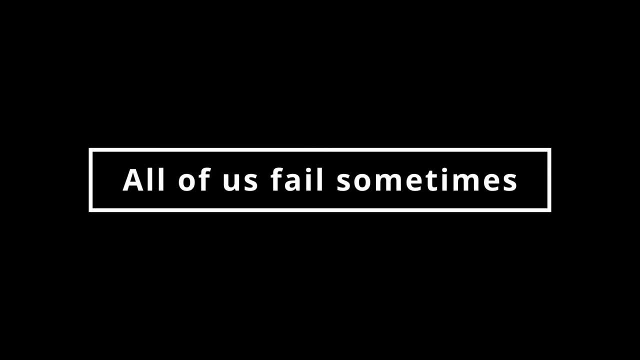 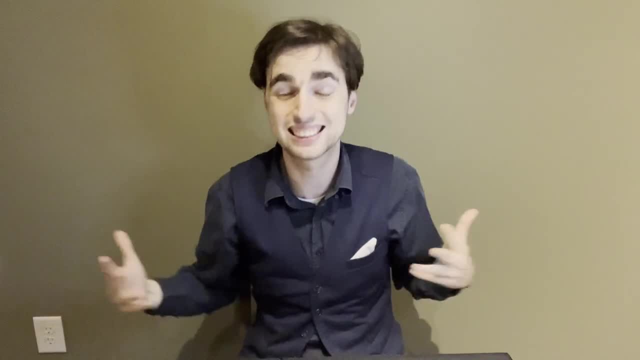 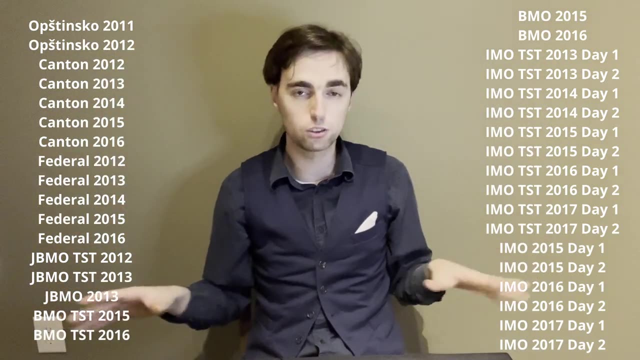 absolutely need to know is that all of us fail. sometimes all of us come short of our goals. sometimes I mean almost all of us. everybody I know has come short of some of their goals at some point, and you might as well. Just to illustrate, here's a list of all the competitions, all the tests. 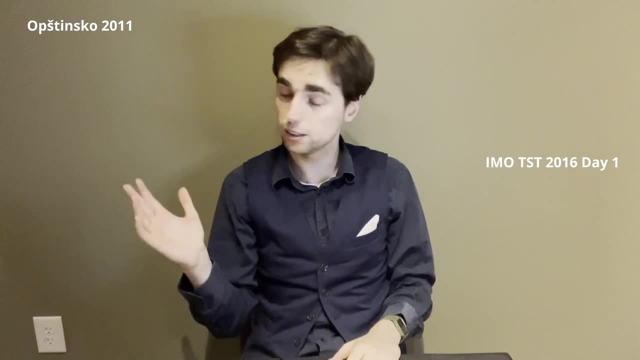 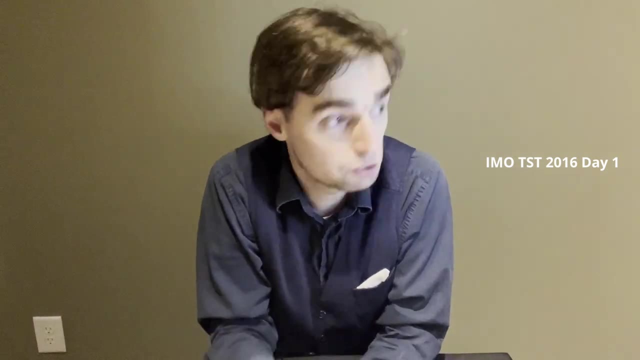 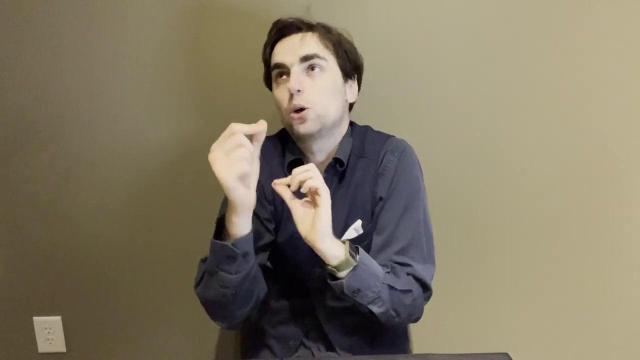 I've actually done in every competition. Now here are the tests that I was actually satisfied with. like it's very, very rare that I was completely satisfied with, and one of them is because I've actually aced the test. but other than that, like there was always another thing that I could have. 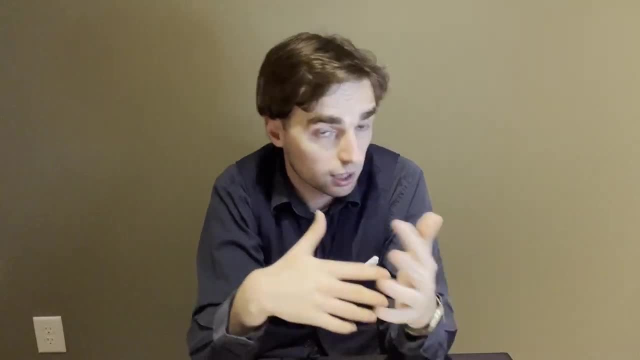 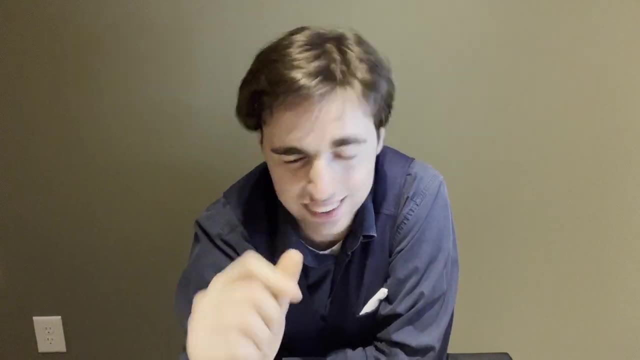 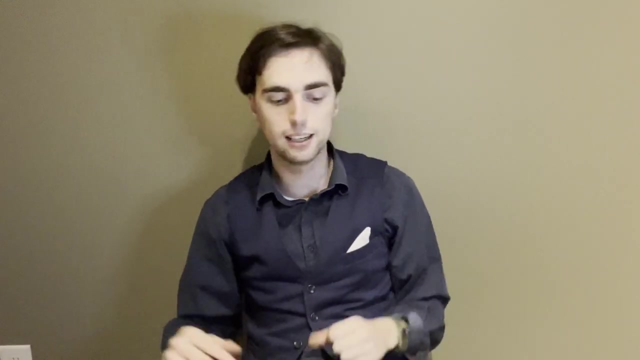 done, should have done or thought I could do better. There were tests where I failed and continued onward, but there were tests when I failed and was devastated, and even devastation has a cost like. one thing that comes to mind is IMO 2016.. I saw that I would get bronze again and I was devastated by the fact. 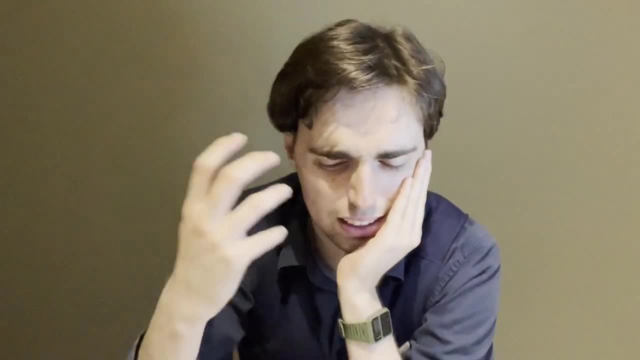 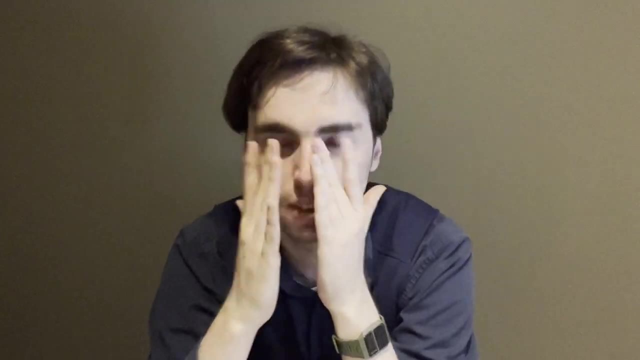 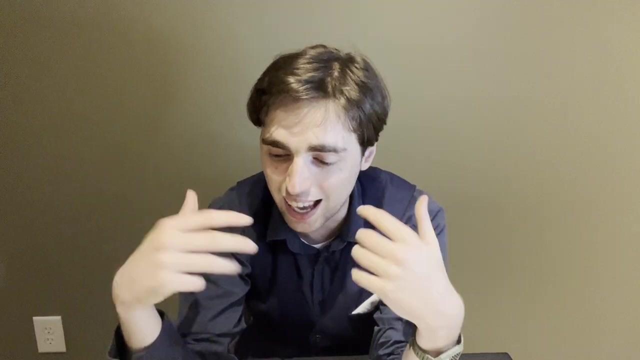 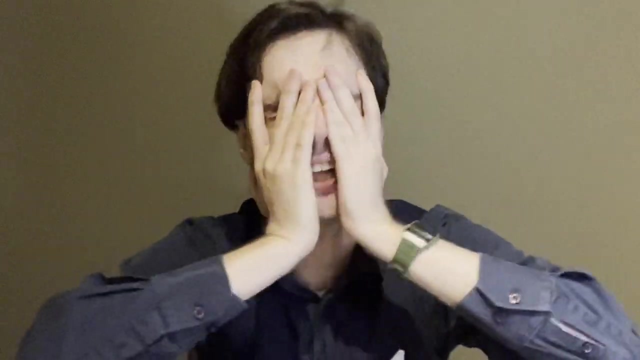 because I was going for something bigger and because of that I was wallowing in my own pity and sorrow like, oh no, bronze, bronze, bronze again, oh. but what ended up happening is because of that wallow and pity and lack of enjoyment, I was so disappointed with this beautiful girl. without that, IMO Now potentially nothing could. 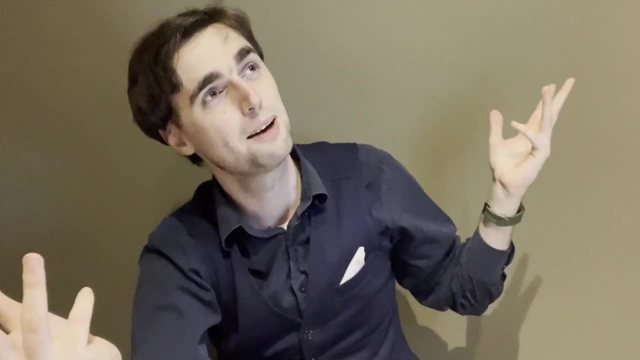 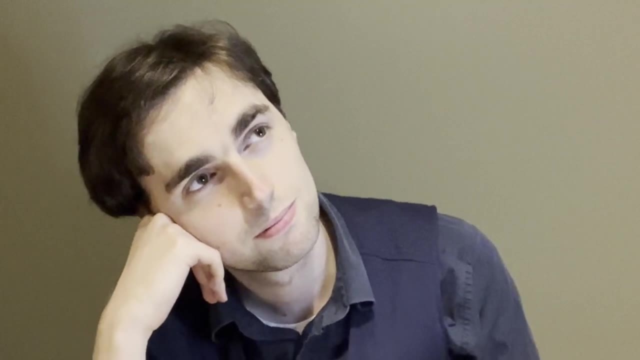 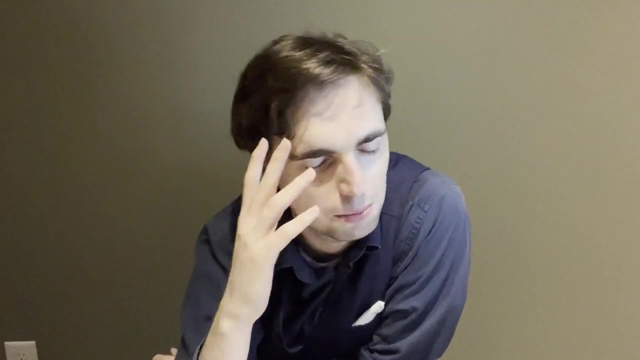 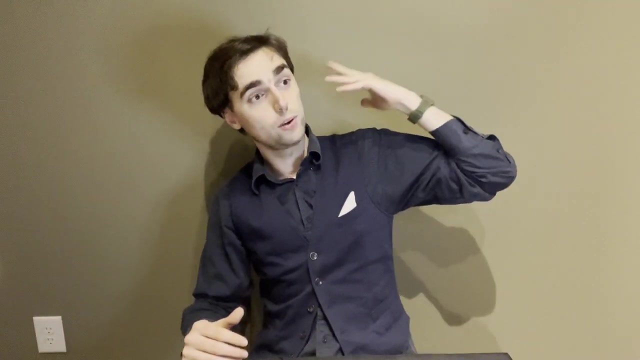 have happened, but there's potentially a slight chance that something beautiful and wonderful could have happened. So note that we all fail and you don't want to wallow in your pity and sorrow. Get on moving something amazing, whether it's going, writing letters to each other or going. 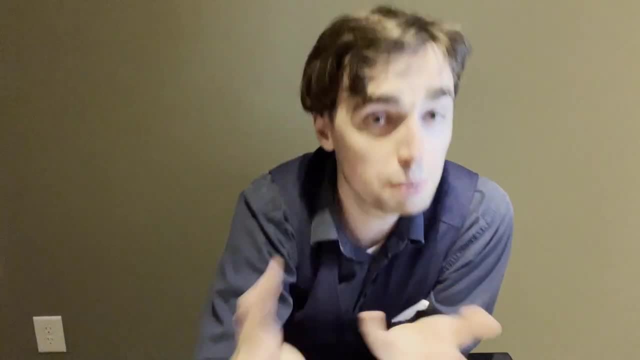 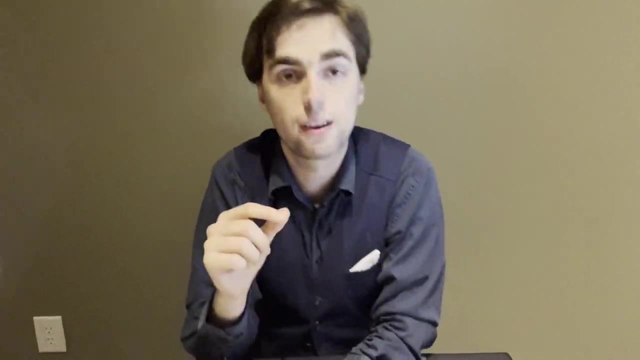 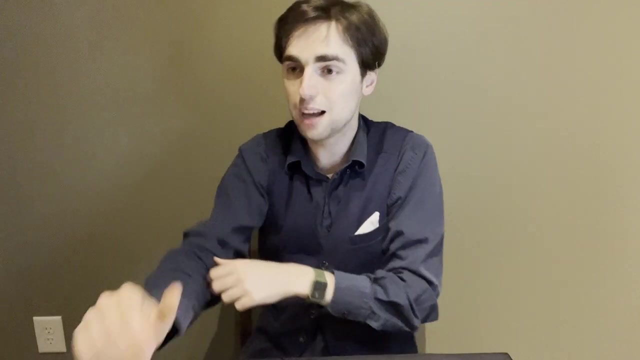 visiting her someplace. oh, my god, you could be missing out on something, so it's okay, you failed. we all fail, which brings me to the next important thing about failure, and that is that one single test does not define you. you know, you're not defined by one single exam. here's a bunch of reasons why you could. 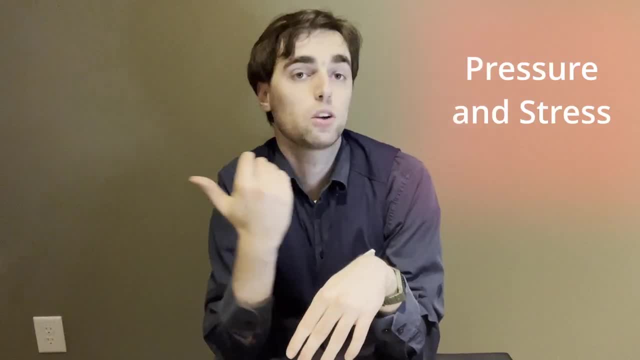 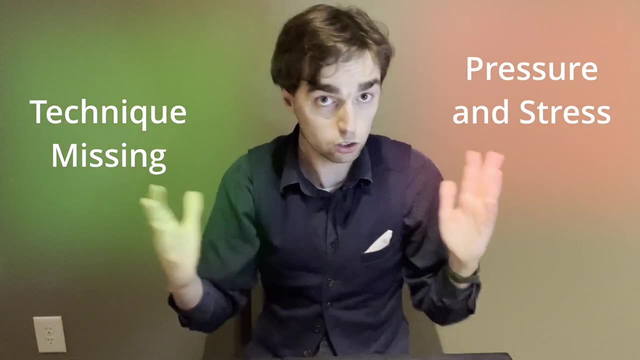 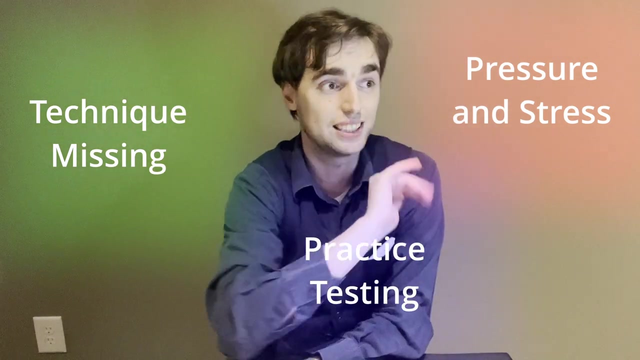 have failed an exam. it could be that you were under pressure or under stress, or it could be that you just didn't know a technique well enough, or it could be that she didn't practice solving problems for a long period of time. and for me I've had a test where the pressure thing has happened, namely my 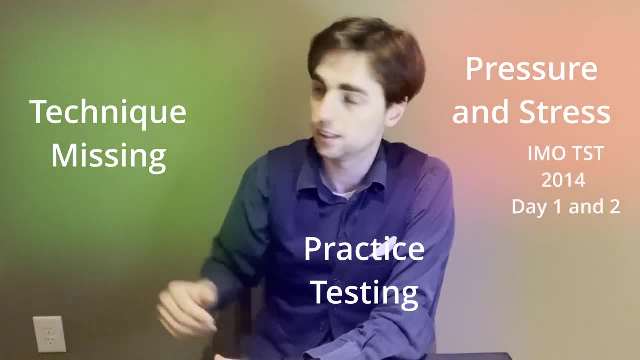 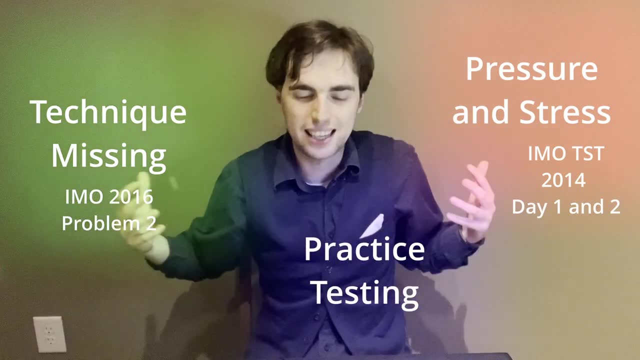 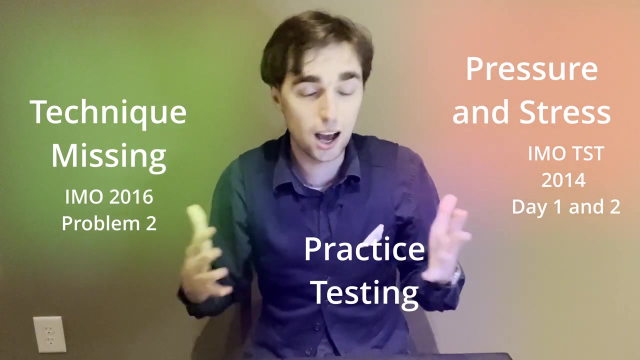 team selection test in 2014. both days I've had an exam where I didn't know the technique. I am the 2016 again problem number two example where I just didn't solved problems for a long enough time. they didn't train solving problems for hours, like I had at the welker math Olympia. 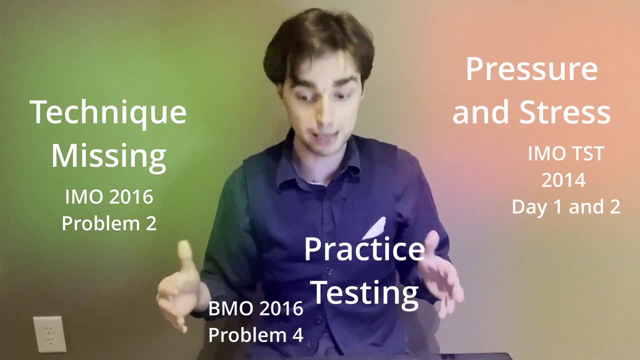 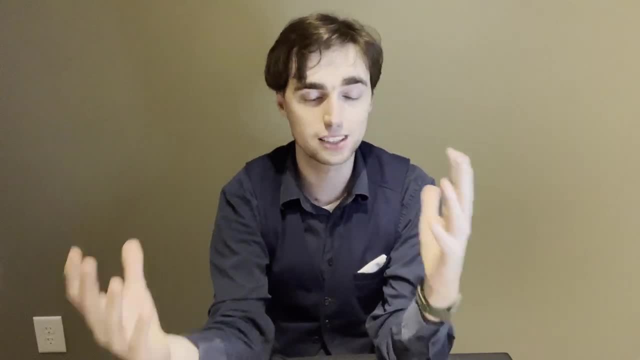 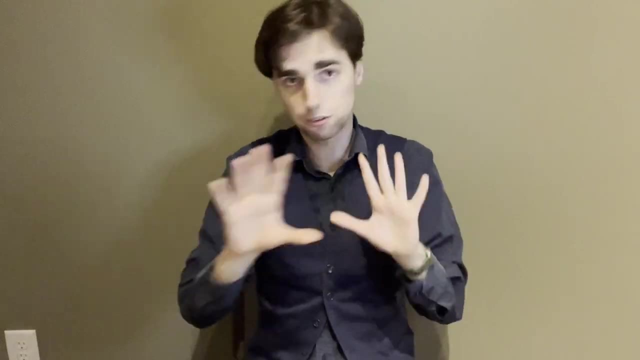 2016, I had three hours for the final problem and I couldn't get anything out of it. why I didn't practice only problems. so, no, there's many reasons why it could have failed and you can fix those, improve upon those over time and next time. now note this: just because you failed an exam does not mean I don't. 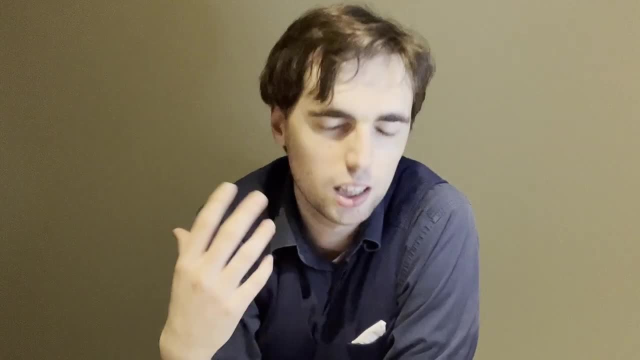 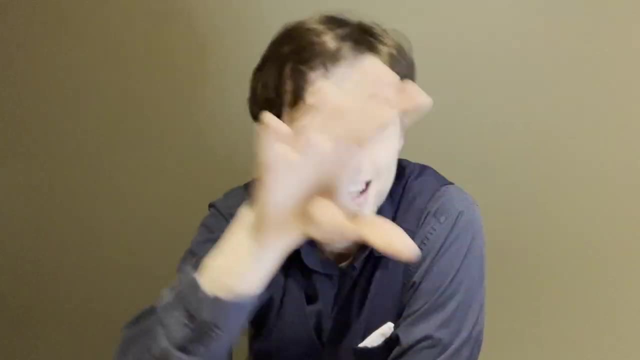 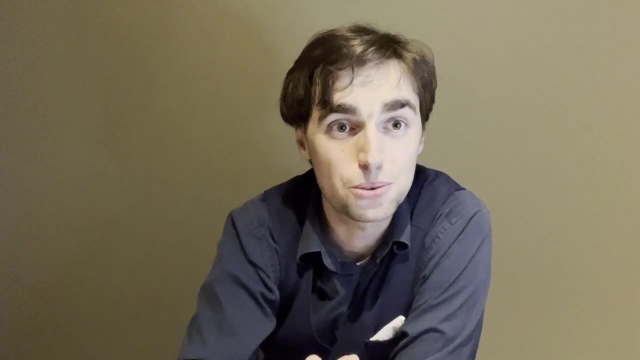 Others won't judge you for it. It doesn't mean others won't call you a loser or tell you that you're not good for that or whatnot. Now, the thing about others calling you a name or trying to evaluate you is that's not your issue. 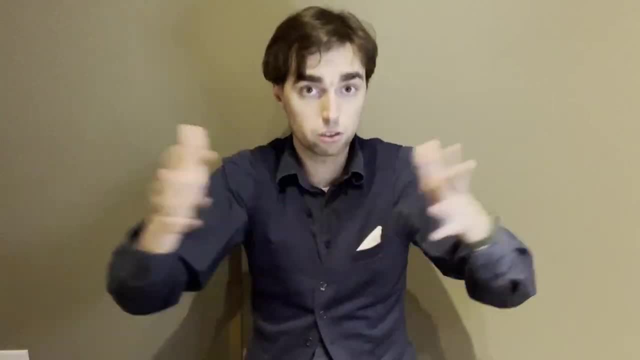 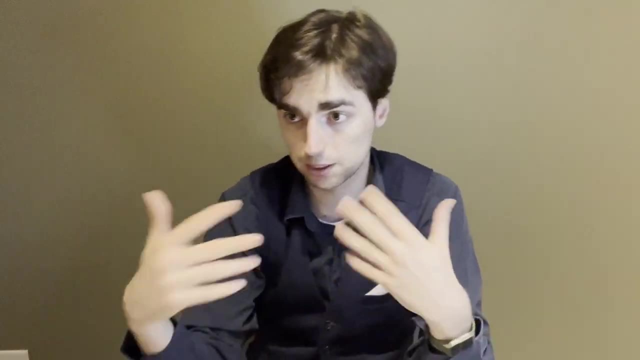 The reason people do use exams is to filter people out when they have a lot of options on who to choose for something, for anything, And so they use an exam as a proxy, as a heuristic- and heuristics are called heuristics because they're not always right- 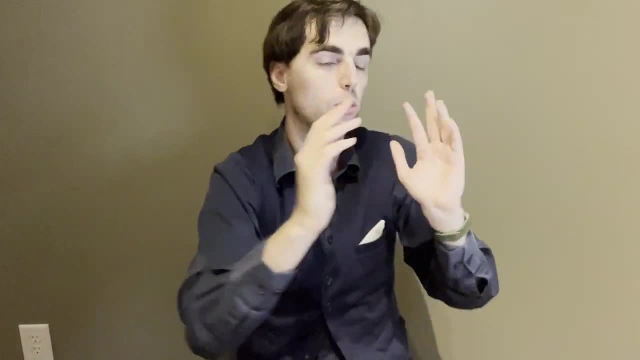 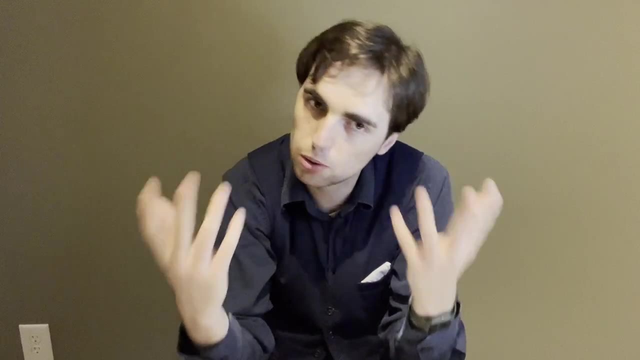 to evaluate: okay, this person I want to work more with or this person I want to work less with. That is that, but it has nothing to do with you. And now, the final and maybe most important fact you need to know is that you can learn, grow and develop yourself. 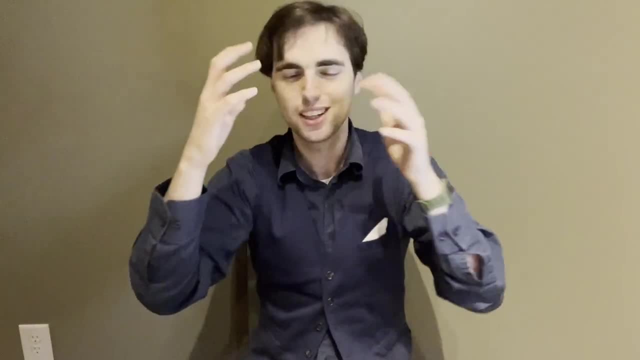 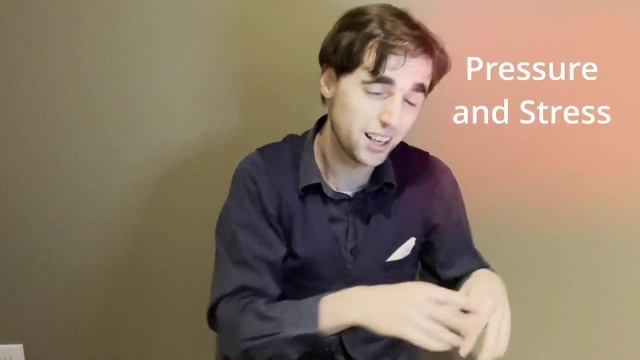 Google the growth mindset, Google neuroplasticity. Know that your brain Can learn, develop and realize that if your failure before was a failure of pressure, you can work on that. If your failure before was a failure of lack of technique, you can learn the technique. 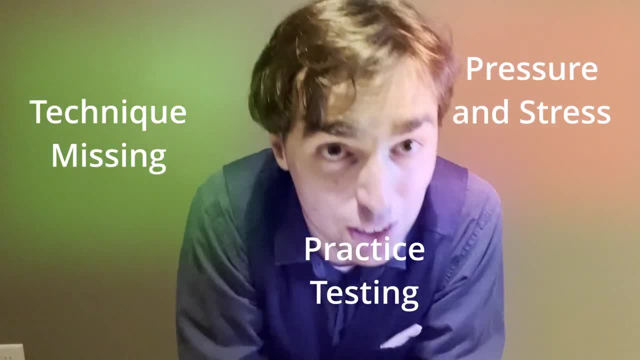 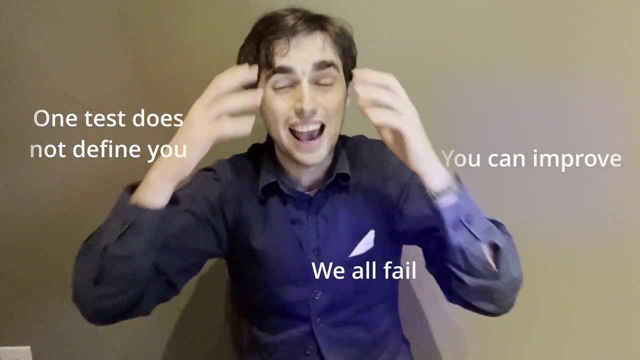 If your failure was a lack of testing conditions, you can test yourself. It's not over. One test does not define you. We all fail and you can grow and develop yourself. Those are the three things you need to know before you even think about should I fail. 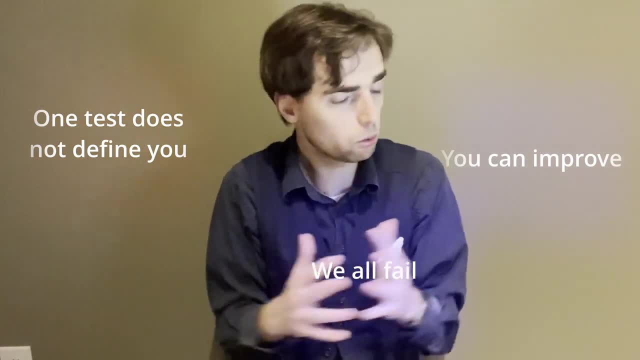 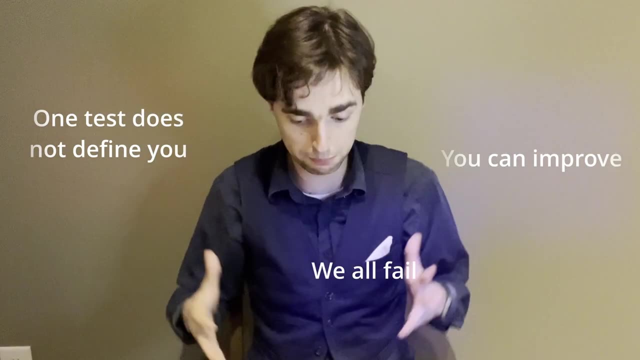 Should I fail? Should I stop or should I continue? You need to know these things first. like that you can grow, that you can become better, that you can learn more, do more, prepare better, deal with stress. It's real. 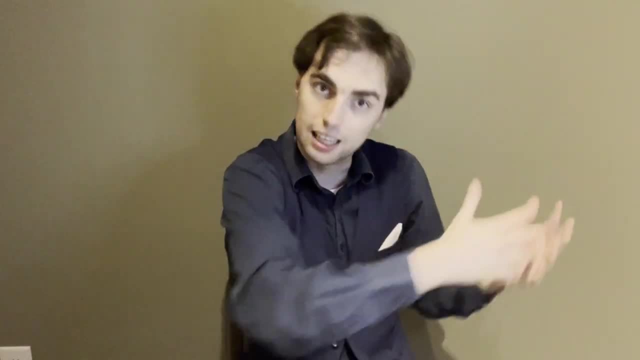 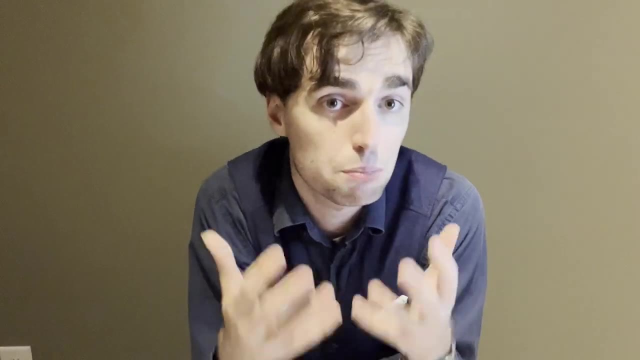 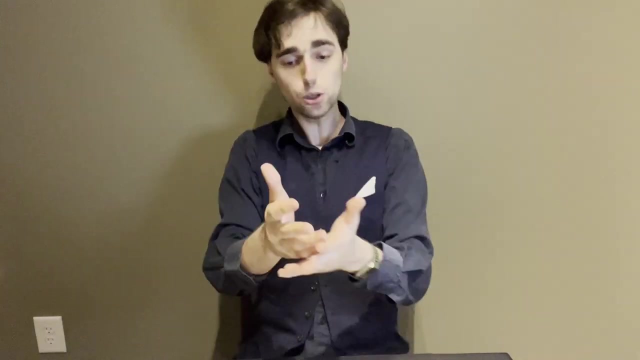 It happens, Exam pressure exists in math competitions, in other exams. Math competitions are an amazing venue for you to learn how to deal with that pressure. And now we move on to the final and potentially most important question, which is say, you decide to continue doing math competitions and a year from now you fail again. 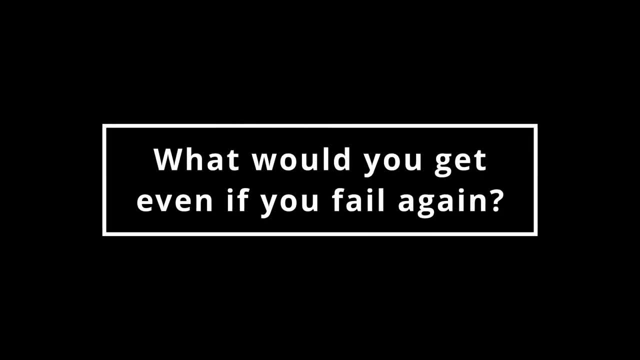 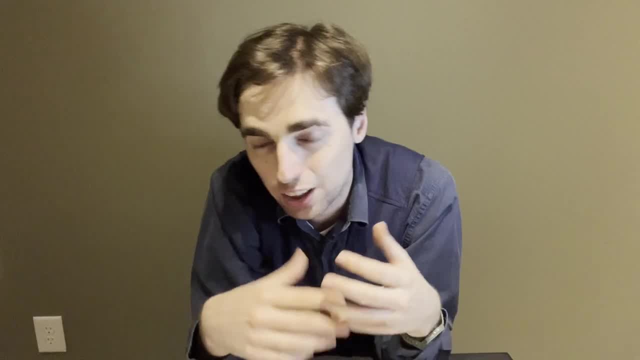 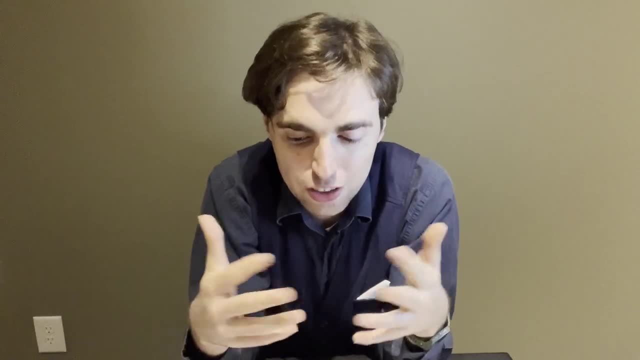 Even if you fail, what is something that you would still gain from math competitions? Now here are some things that I can tell you that you will get if you decide to really devote yourself to this: learn, learn, learn and try to get better in all these areas. 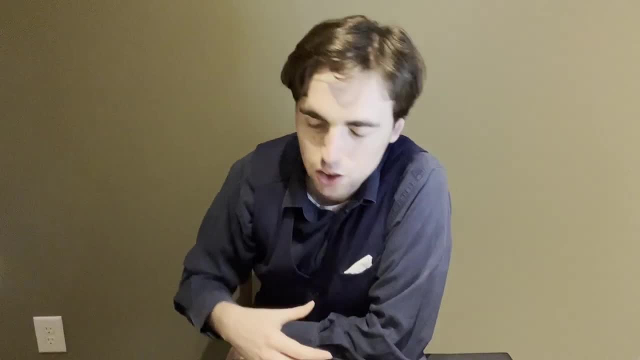 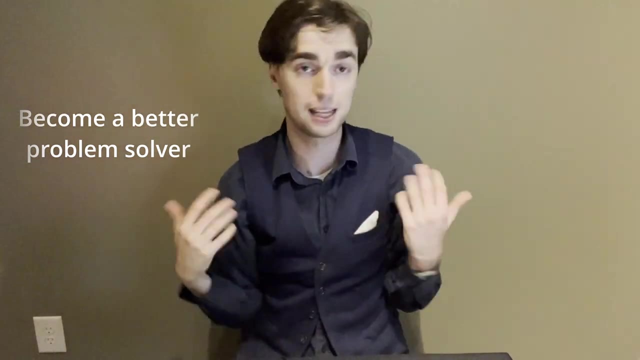 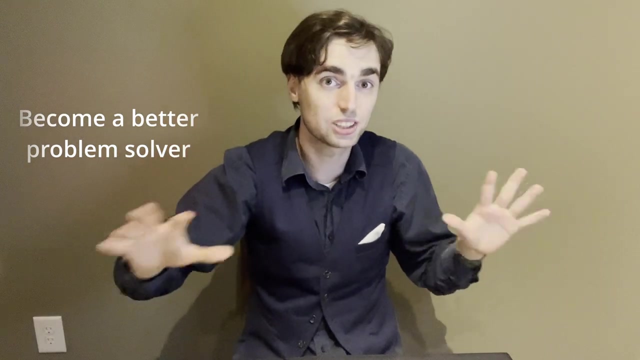 If you find these weaknesses, improve upon them. Namely, you will become a better problem solver, Solving problems that don't have obvious solutions, that aren't just applying techniques. you're going to become a better problem solver Now. it is helpful to have that habit in other areas of life that you may go into. 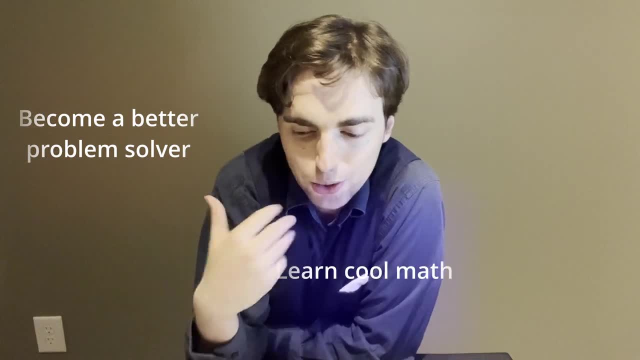 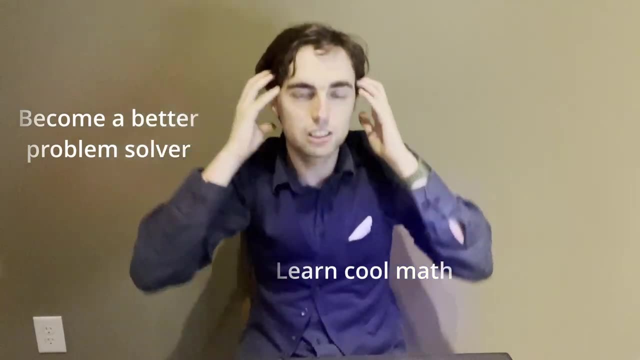 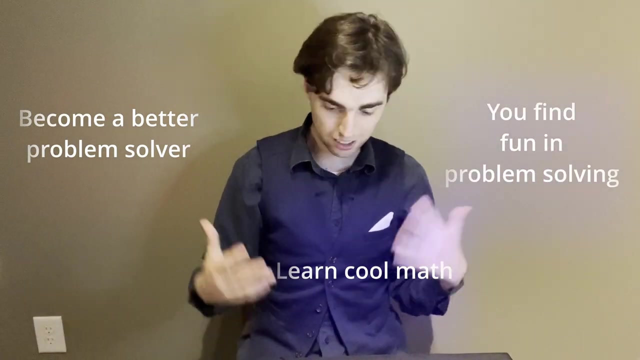 The second reason you might want to do this is you're going to explore and learn cool math, even if you fail. You can fail, But the knowledge, The knowledge still stays with you. Or it could be also that you just enjoy problem solving, that you find it fun that you have. 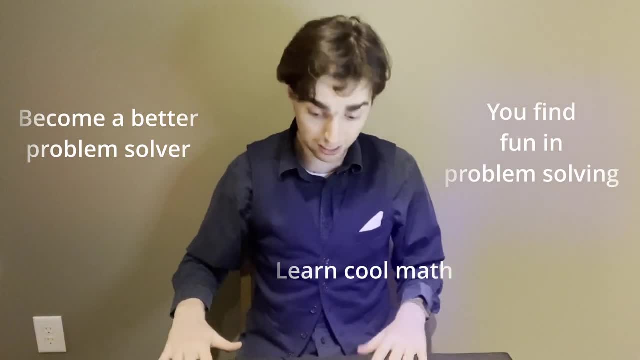 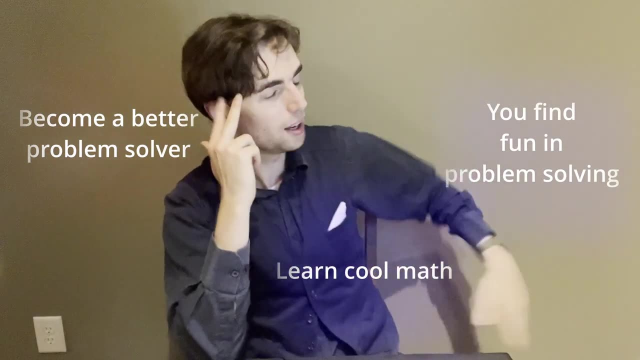 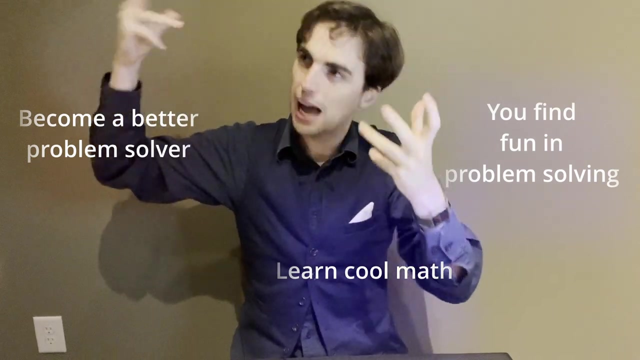 gratitude that you're able to learn and develop yourself and learn these pretty cool things and how they work. how, wow, you prove stuff with that. What, How, What are the inner workings like? How does math work? What are the connections to everything? 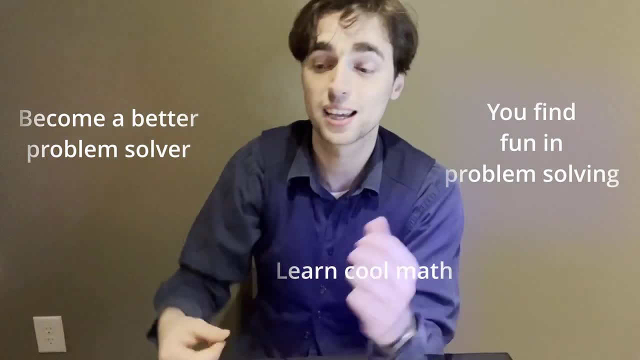 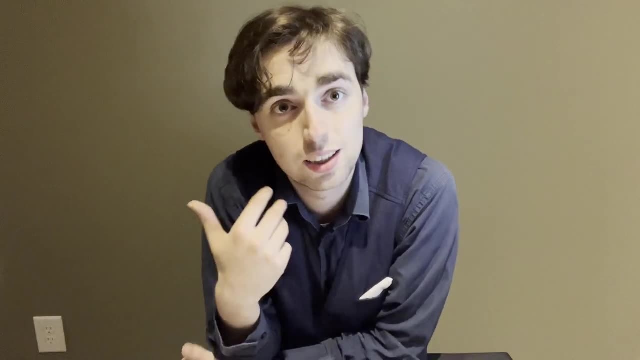 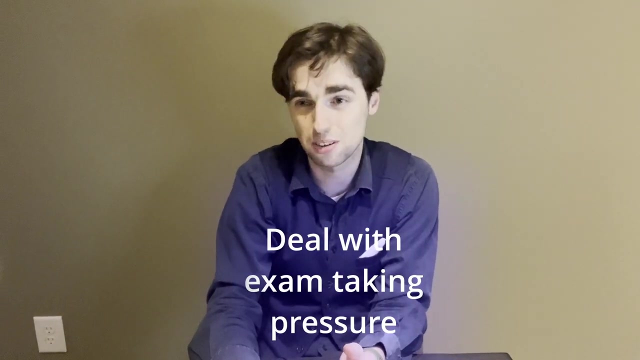 It is very cool. It is very cool. You learn yourself to feel that. And finally, something I actually appreciated only after the fact is, by taking exams under competitions, is you learn how to take exams in general. You learn how to deal with pressure of exam taking. 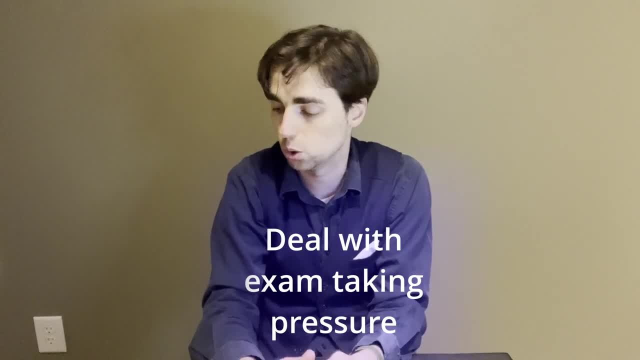 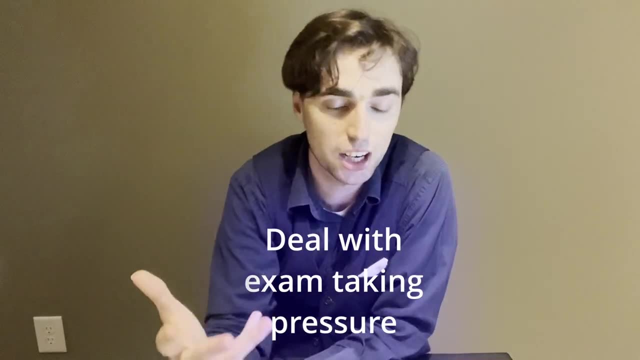 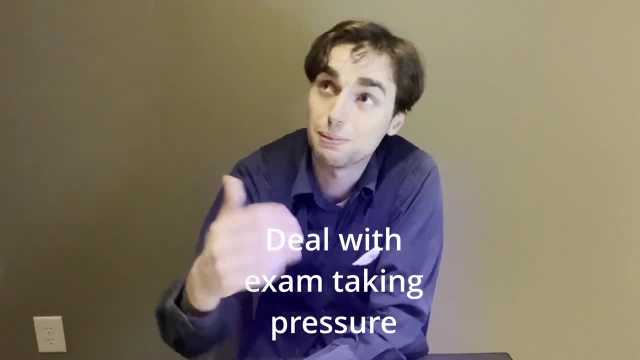 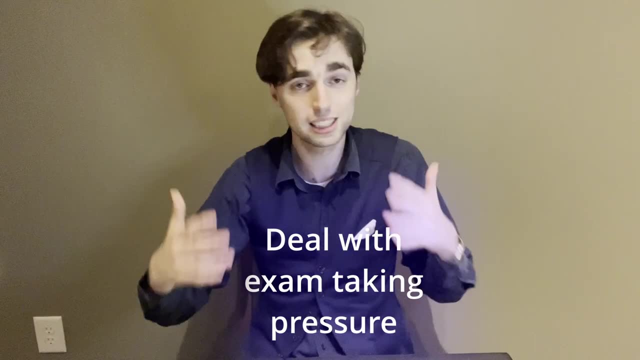 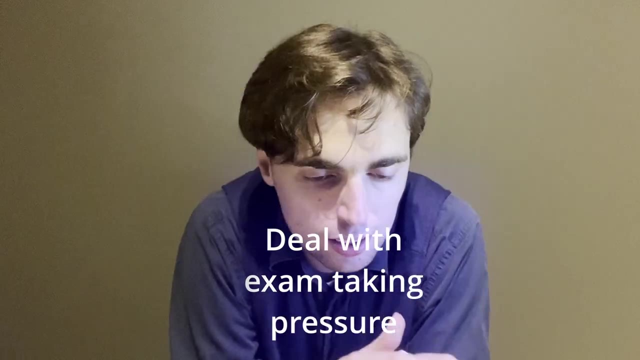 If you learn how to deal with the stresses of that and the expectations that come with that, you'll be able to better deal with tests and expectations and all the pressures that come with taking tests in a university setting or preparing for something where you need to present. 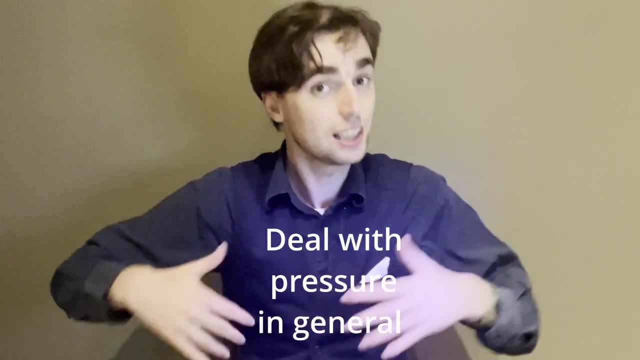 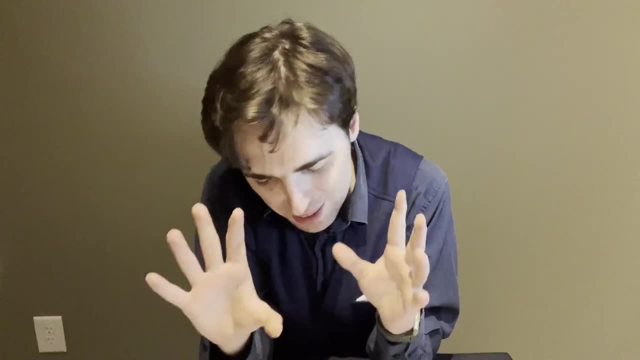 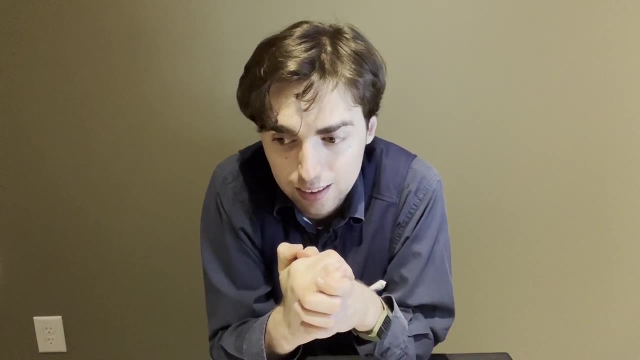 This is the thing where, if you learn how to deal with pressure here, you can learn how to deal with pressure in other areas of your life, and this can be useful for you wherever it is you end up. And now the final thing, which is something I actually didn't know until later, is that 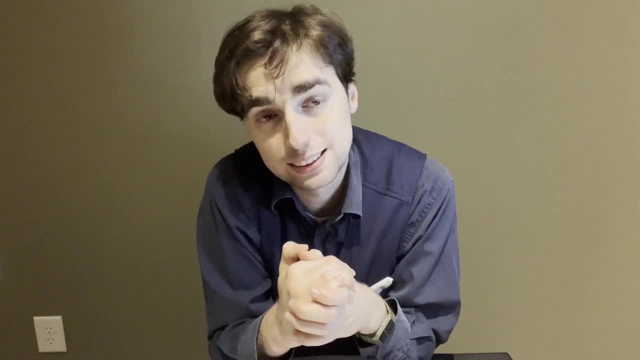 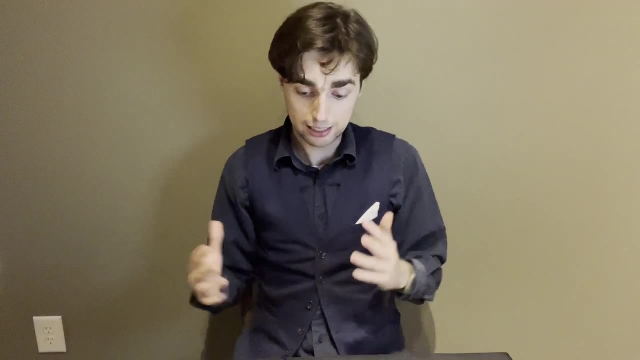 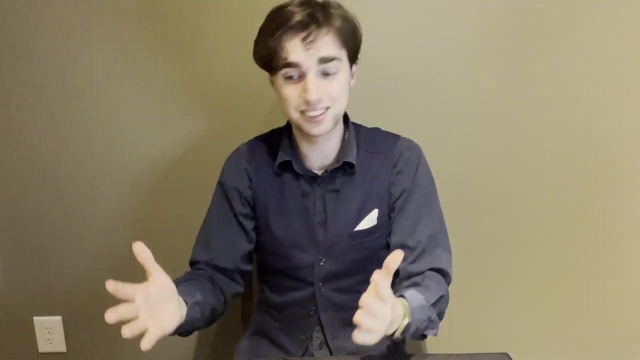 a good reason for why you want to do competitive mathematics is because this can be your ticket to the best universities in the world. I did not know this was a fact until after I had gotten a bronze medal, But if I had known, I would have definitely definitely done more competitive mathematics.